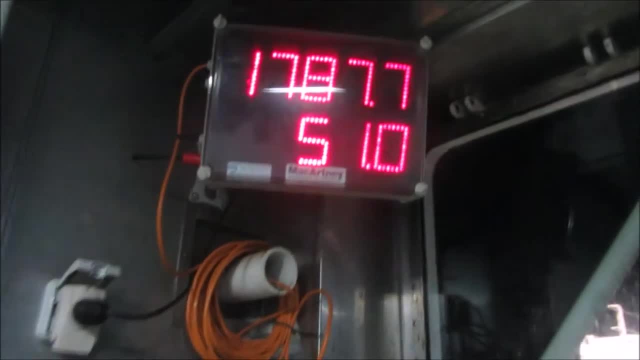 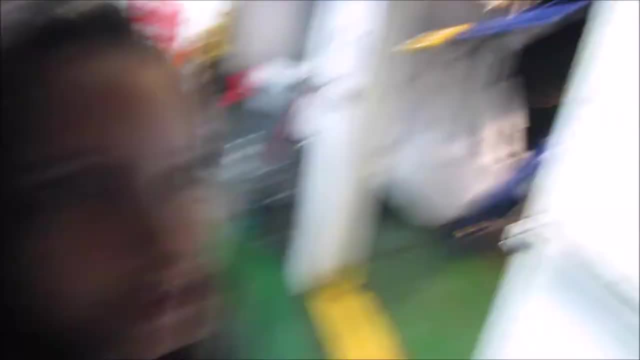 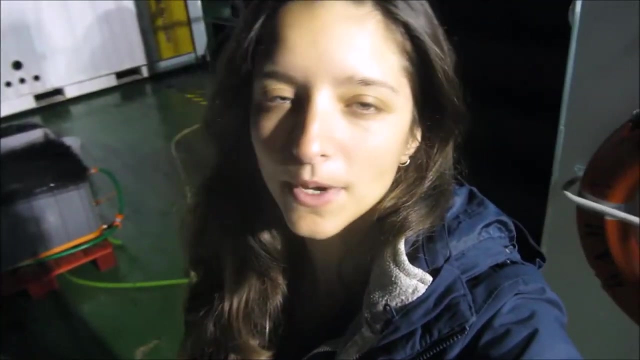 Here you can see the depth at which the CTD is now 1,785.83,. well, it's always. it's coming up now, so of course it's always changing. There's always one first drop. We are the first person in the CTD room and we always do station when we arrive on station. 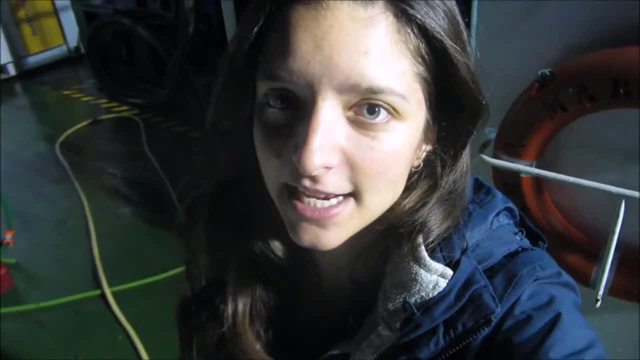 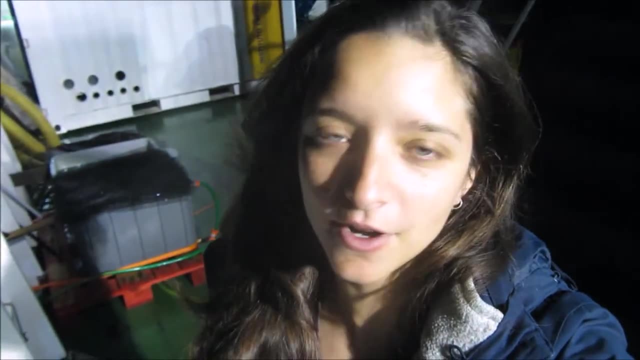 it doesn't matter what time it is of the day. it can be in the middle of the night, it can be in the morning, it can be during in the middle of the day. we sample because we have a limited time for a limited for a certain number of stations, so we have to make maximize. 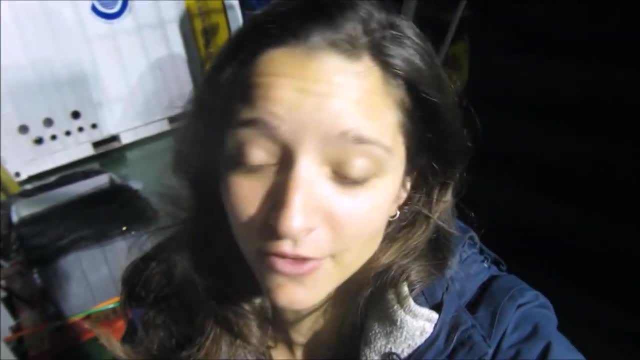 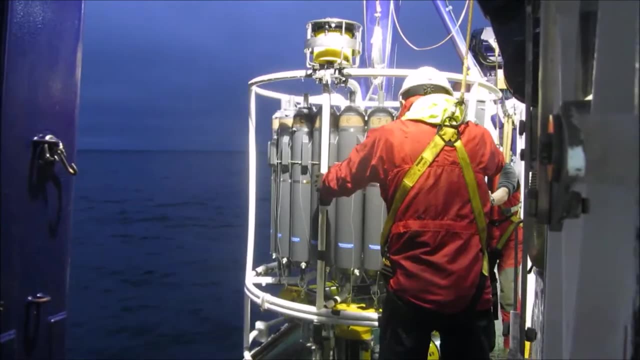 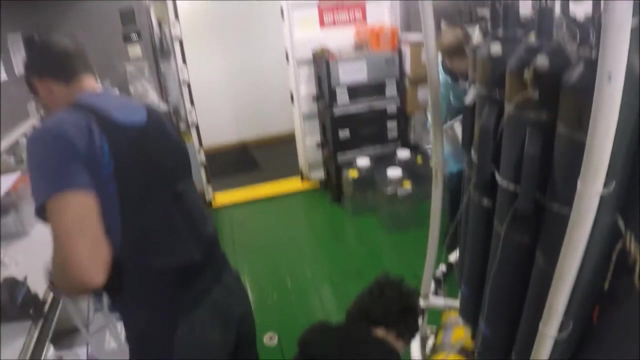 our time, and for that we have to sample whenever we arrive on station, And now we just need to wait that it's up and then sample. It is on deck. Once the CTD is back on board, the scientists collect water from their pre-assigned miscan. 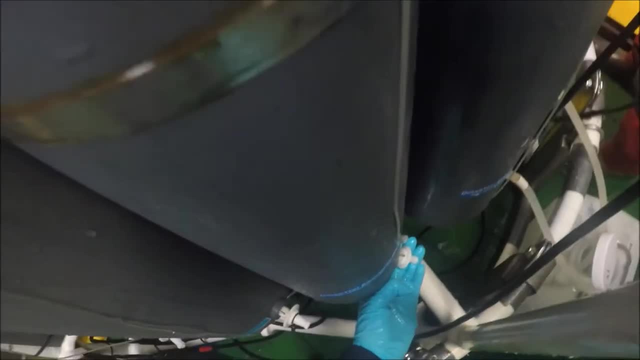 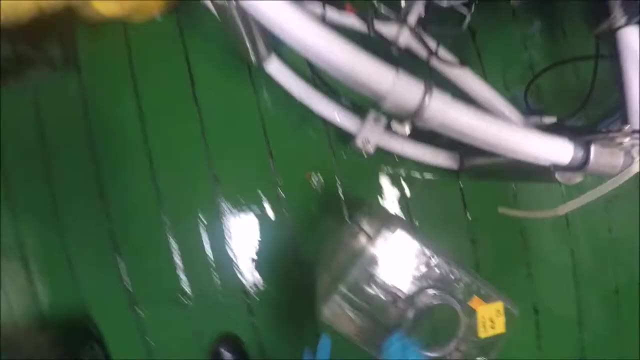 bottles with water from the depth they want. In our case, we collect water to study different parameters at different depths, such as bacterial abundance, microbial community composition, methane concentrations, and we also collect water for some extra experiments. After all, water has a great impact on the body. 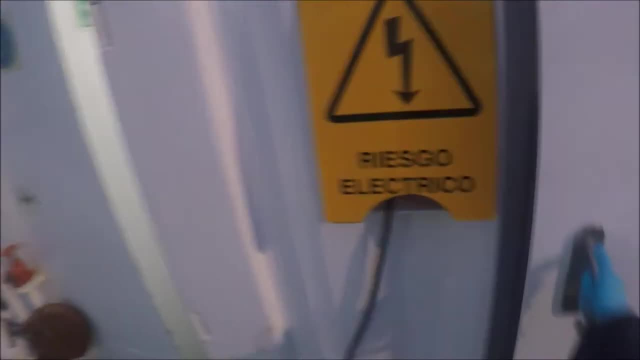 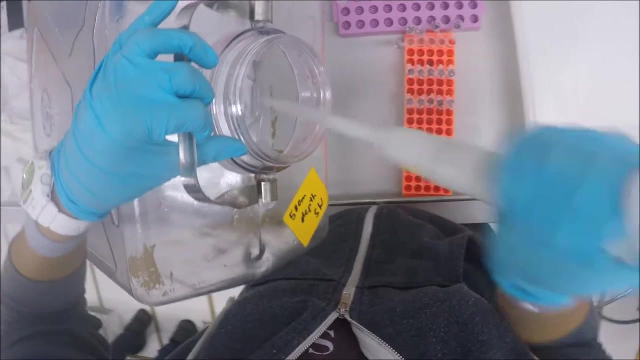 It's a very important part of the body. It's a very important part of the body And once the water has been collected, we proceed back to the lab and continue doing lab stuff, such as filtration experiments and lots and lots and lots of pipetting. 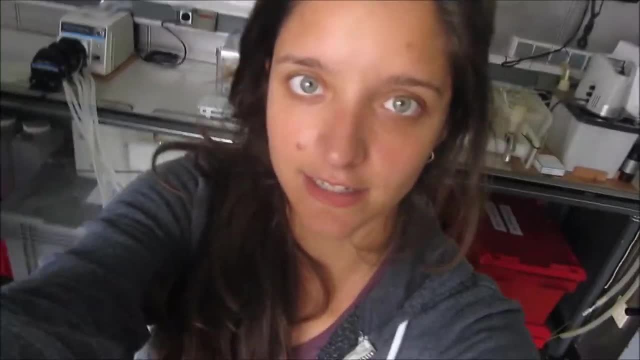 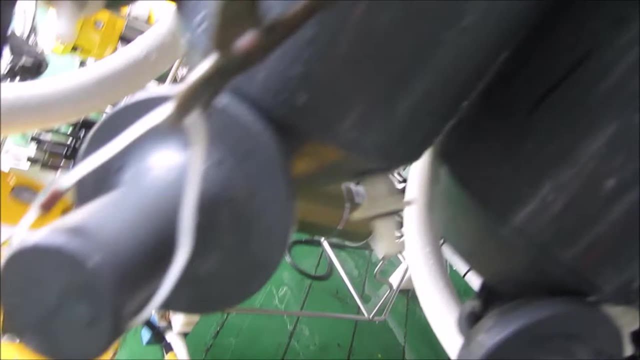 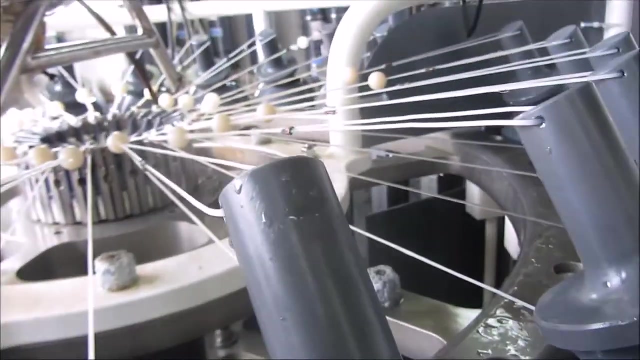 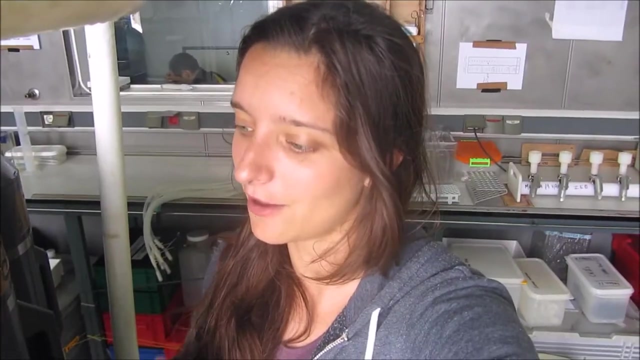 We will send the CTD down again and, as you can see here, the bottles are open, up and down and connected to this structure in the center, and then from the computer we can decide when to close each bottle, and then we have water from whichever depth we want. So we will put the CTD down again, We will send the CTD down again and as you can see here the bottles are open up and down and connected to this structure in the center and then from the computer we can. 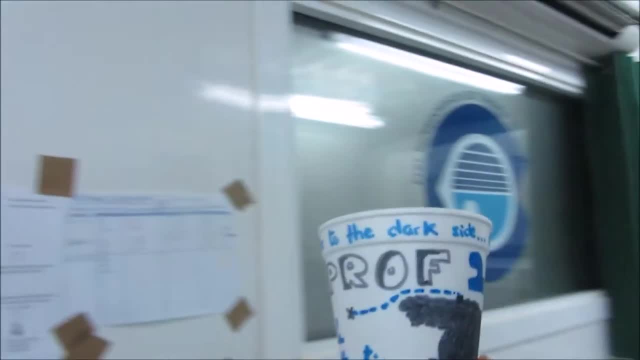 decide when to close each bottle, and then from the computer, we can decide when to close each bottle, and then we have water from whichever depth we want. So let's go back to the lab. tomorrow we will see what happens after we take the mask off. 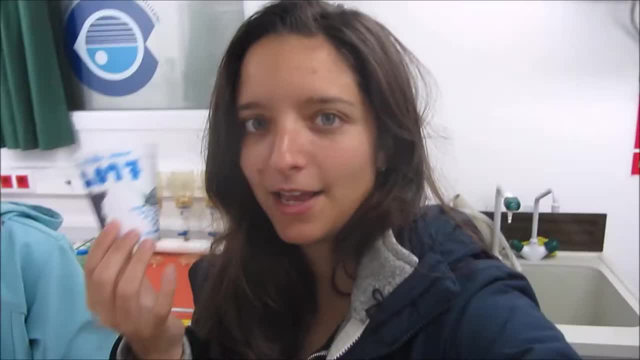 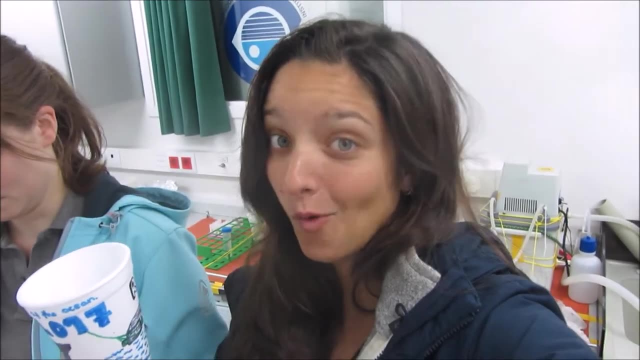 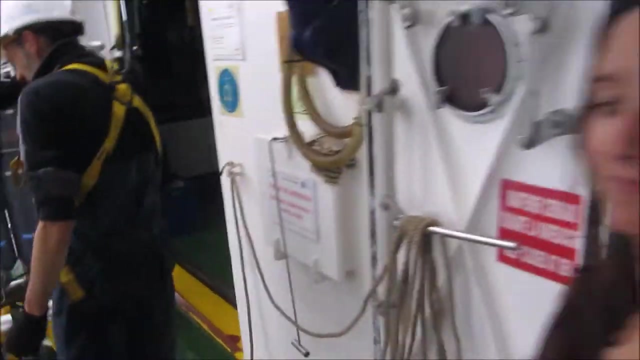 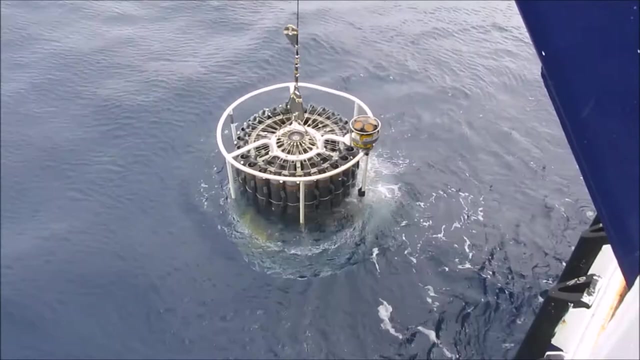 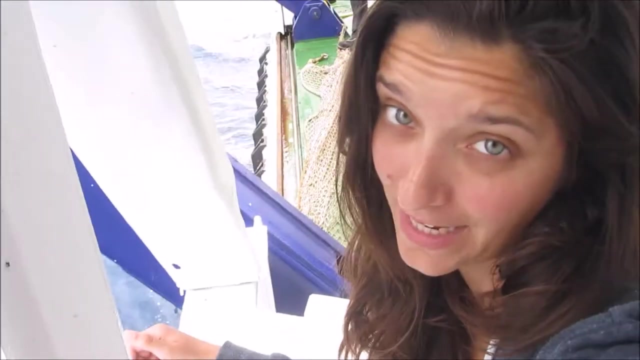 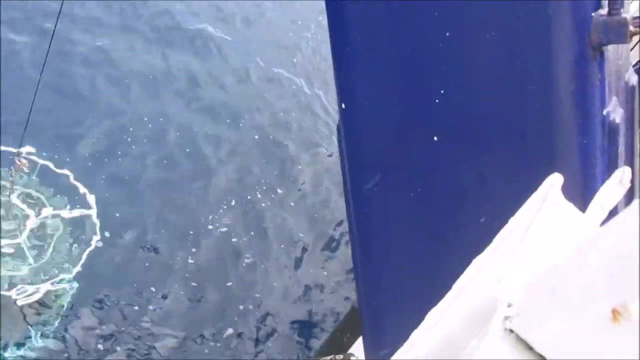 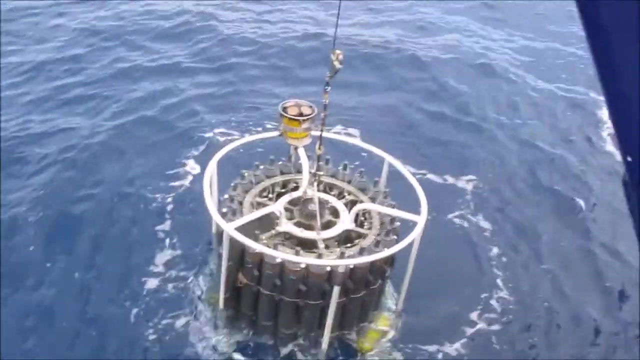 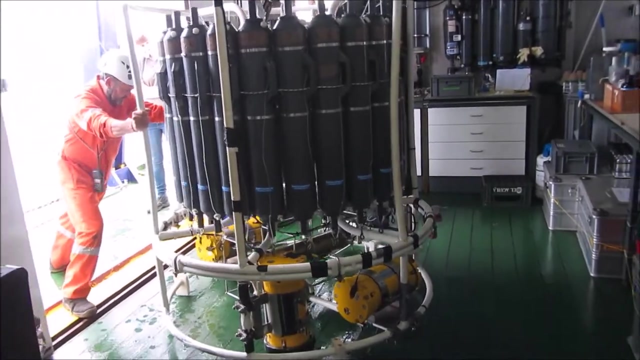 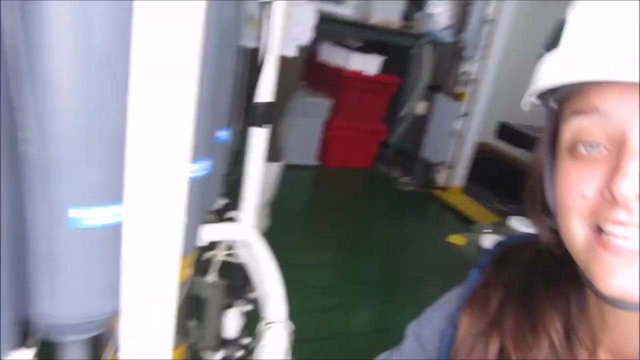 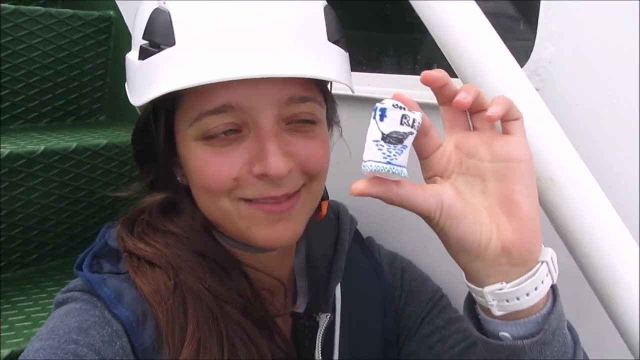 the CCD. Thanks for being with us today. We will see what happens with the test tube. Oh thanks, After 3 hours it's coming back up. So who can guess what happened to our cups? They look super tiny And you know why. 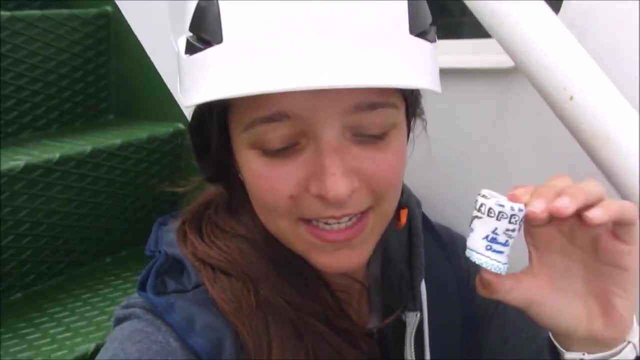 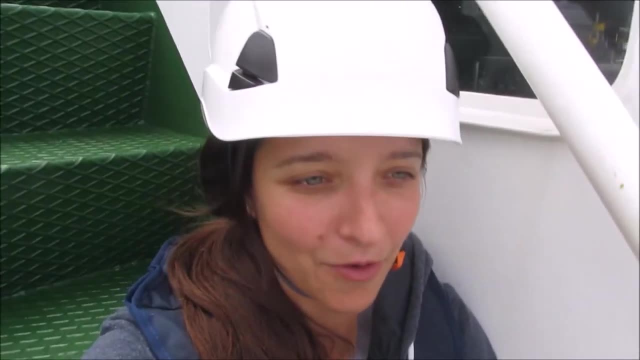 Basically, the cups that we put on the CTD were full of air, so they are made of styrofoam, which is a type of plastic which has a lot of air. So, of course, under pressure, all the air comes out of the plastic and there's no air left. 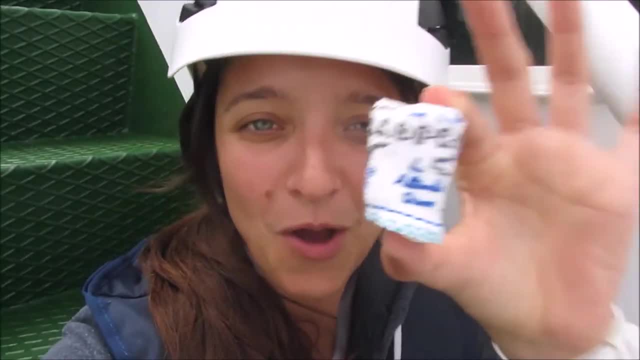 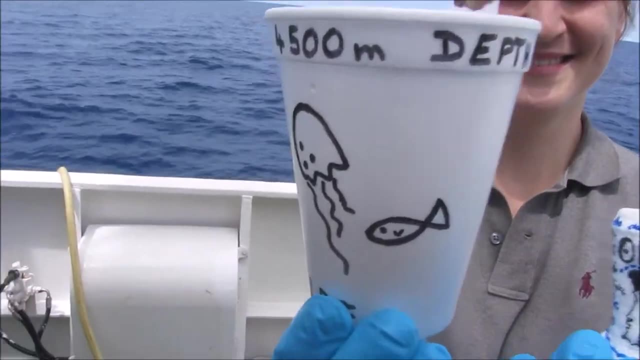 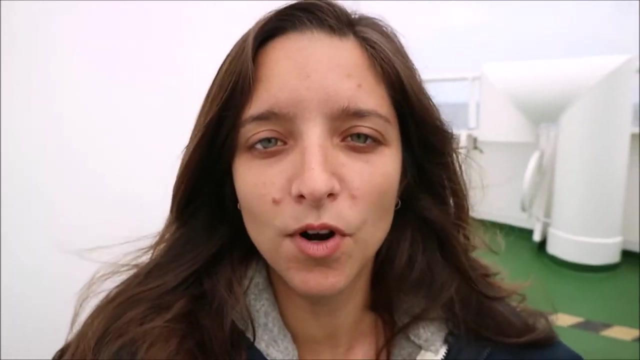 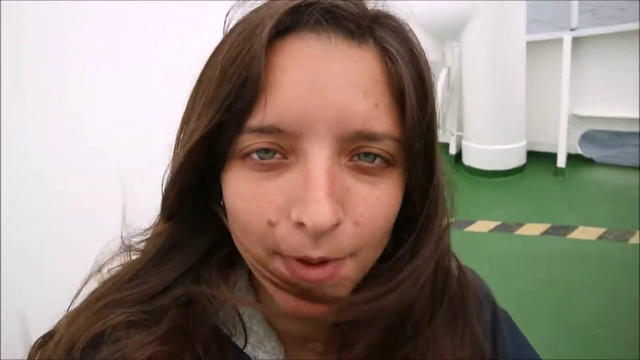 So it just becomes very dry, Very, very small and compact. And look how cute and small it is. All these parameters and many more that I did not talk to you about. we are capable of characterizing different water masses over time in different parts of the world. 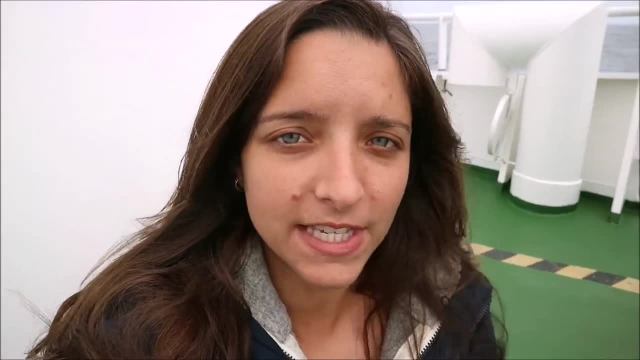 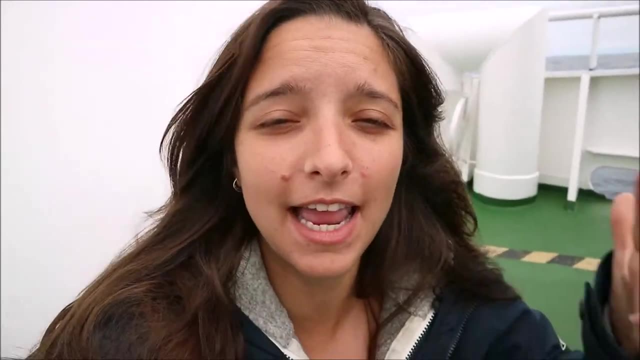 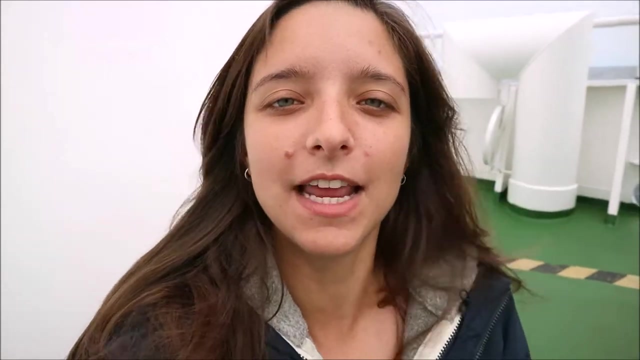 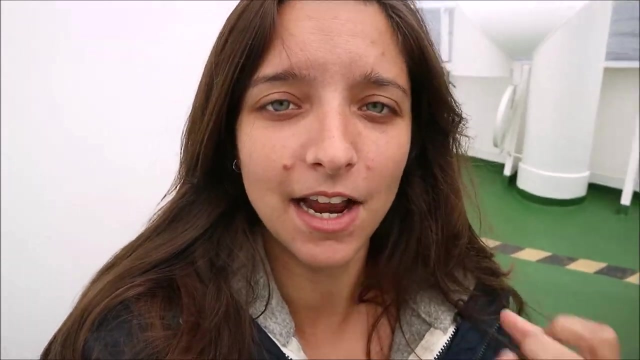 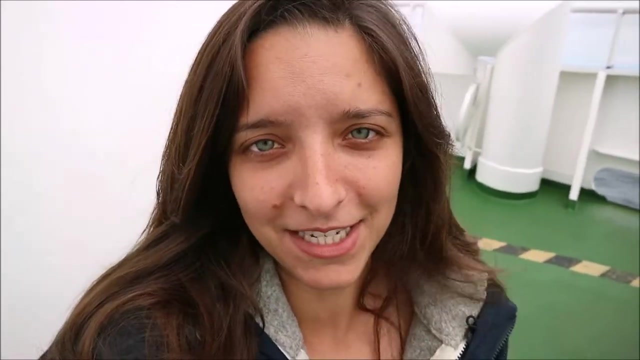 And this takes us one step closer into understanding how these complex systems work- Biologically, physically, chemically, geologically- which all interact with each other and allow us to have the world that we have today, Because, ultimately, the ocean is a very important player in maintaining our world's climate and our world's atmosphere, and maintaining the world as it is so that we can live on it. 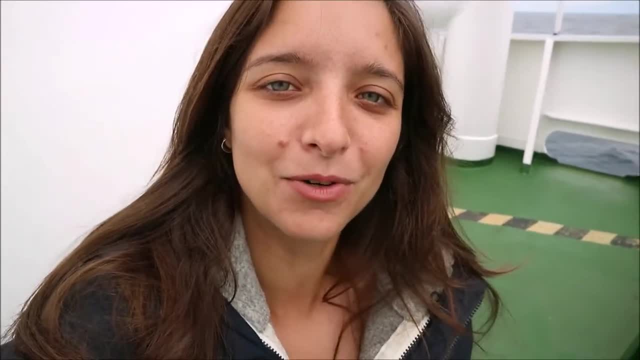 This is it, guys. I hope you learned a bit of some things that we can do here on the cruise, And thanks for watching.